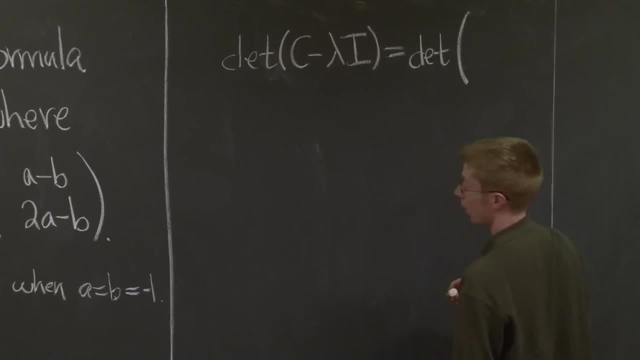 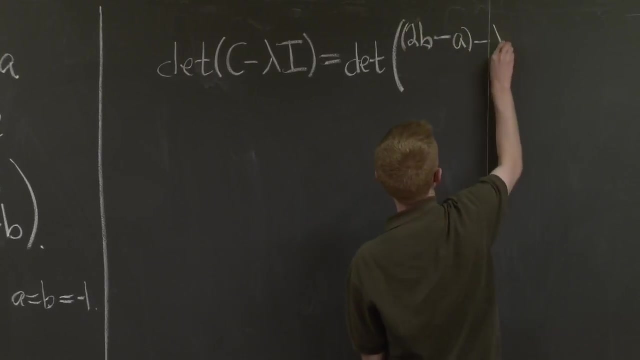 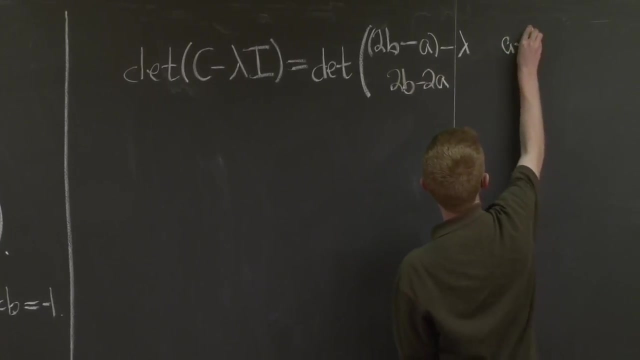 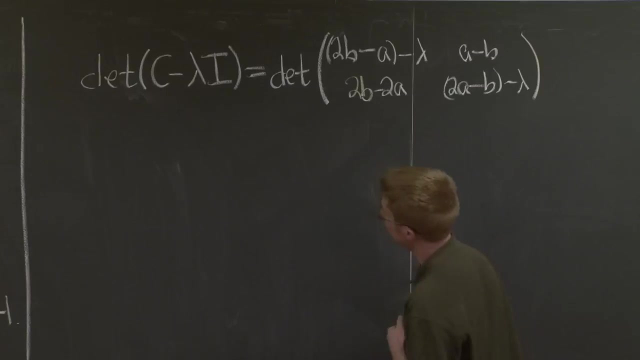 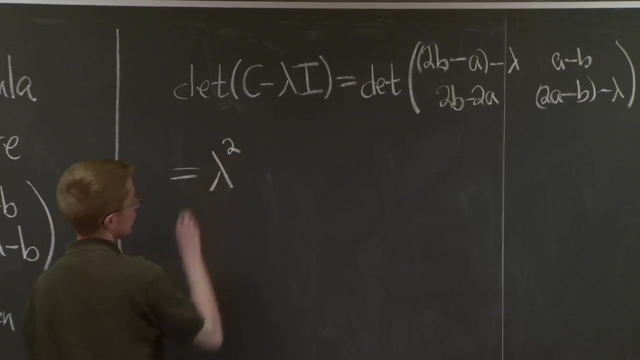 which is just the determinant of this matrix: 2B minus A minus lambda, 2B minus 2A, A minus B and 2A minus B minus lambda. OK, If you compute this well, we have a lambda squared term. 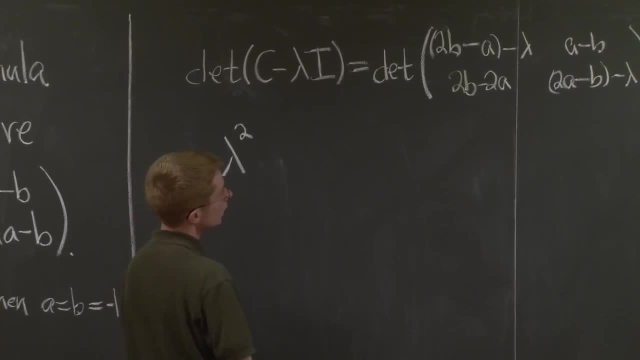 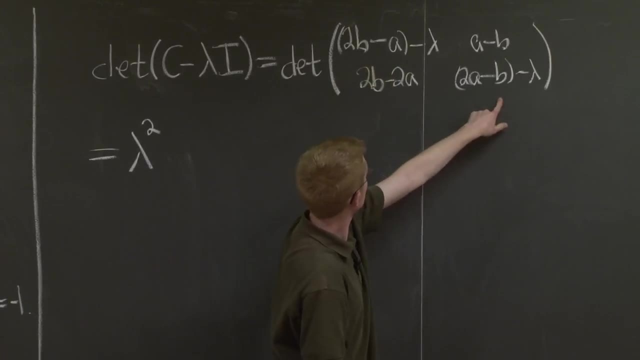 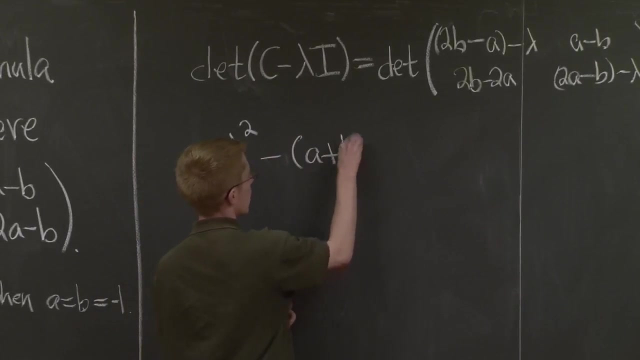 OK, Our lambda term. If you look at it you'll see we get 2B minus A plus 2A minus B, which is just A plus B, and we have a negative sign That's negative A plus B times lambda. 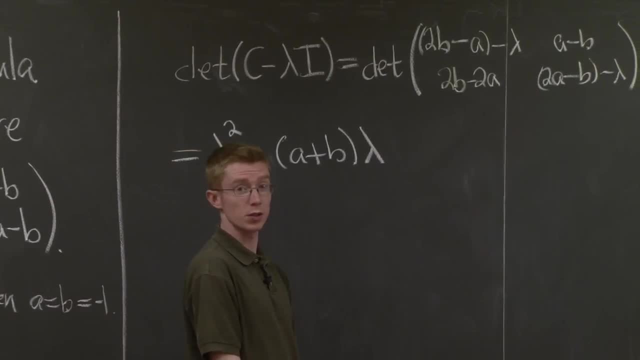 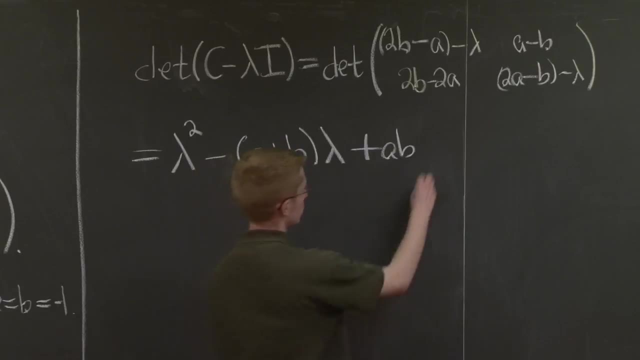 And our last term is a little tougher to compute, so I'll let you do it yourself. But you're just going to get plus AB And this will factor as lambda minus A plus lambda. OK, So this is A times lambda minus B. Good, 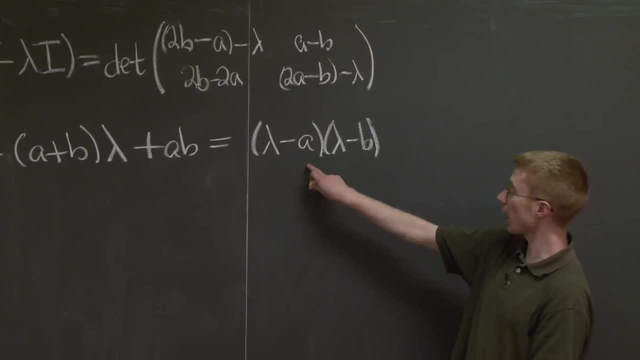 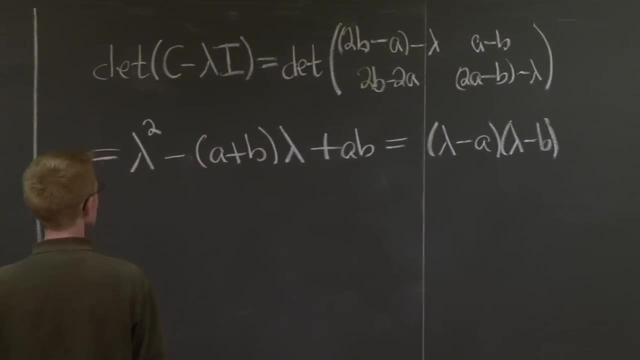 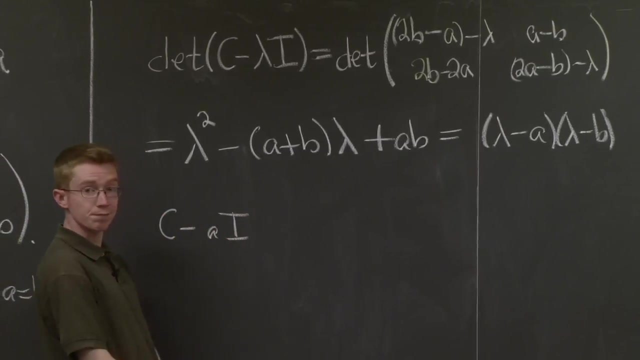 So our eigenvalues are just A and B. OK, Now we need to find our eigenvectors. So how do we do that? Well, what we need to do is we need to look at C minus A times the identity, And we need to find the null space of this matrix. 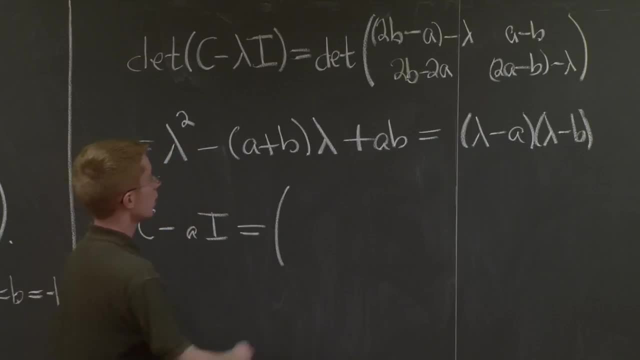 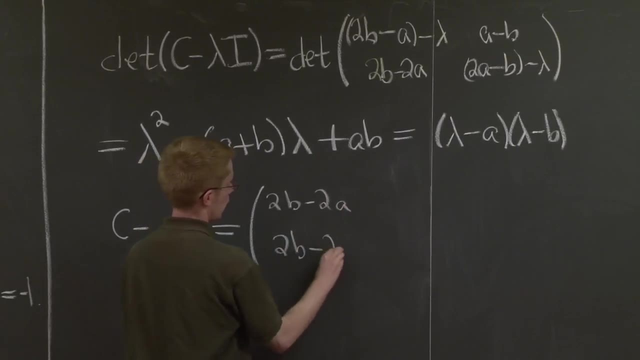 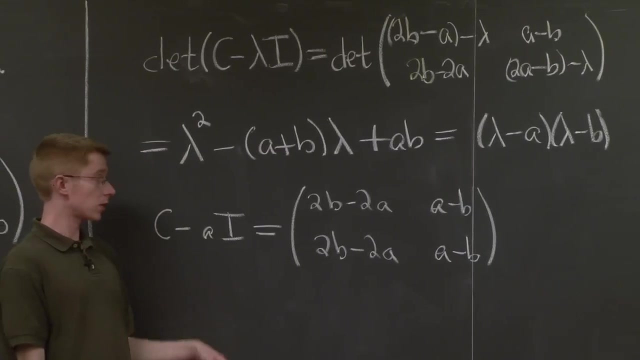 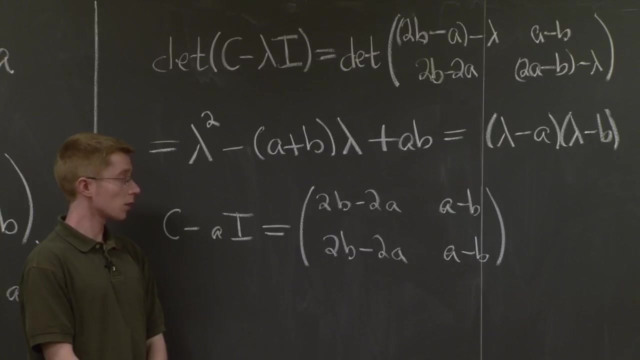 So what do we get here? Here we get 2B minus 2A. and then our next entry: here we get 2A minus B minus A. So this is A minus B. Good, So you can see that this matrix has the same columns. 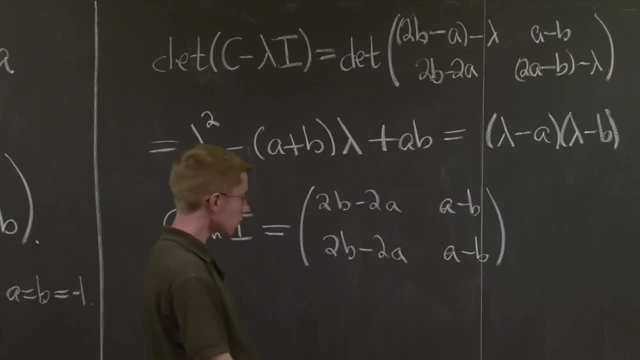 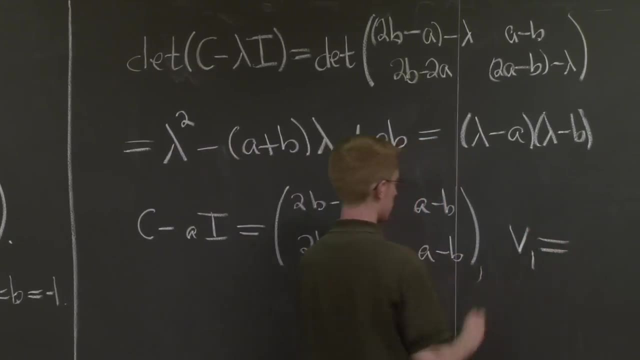 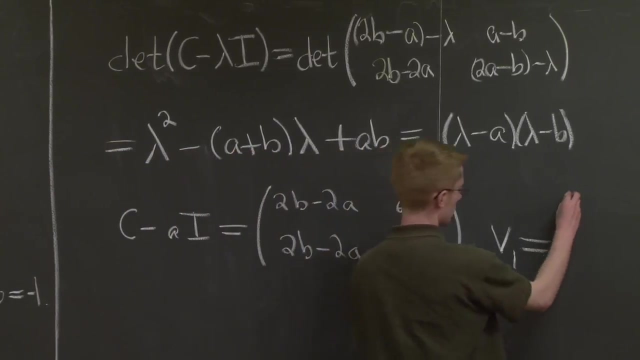 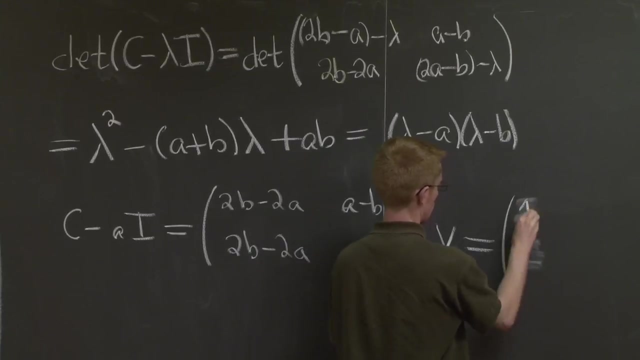 And this the same rows, And so you can see that a vector in the null space. since this column is negative 2 times this column, we can see that our first eigenvector is just or 1, 2, I should say 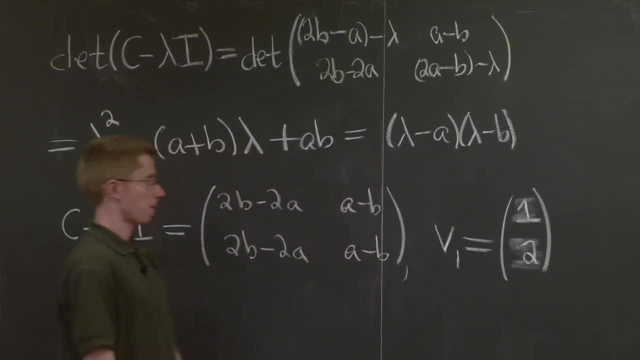 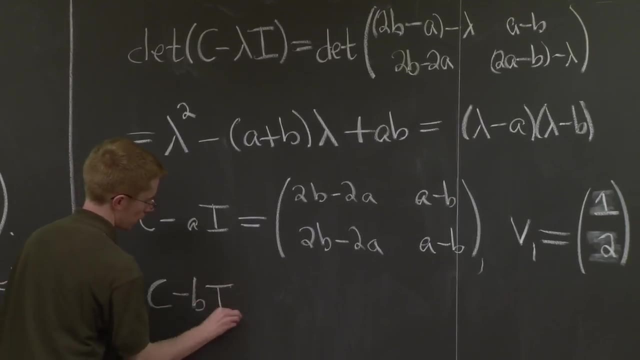 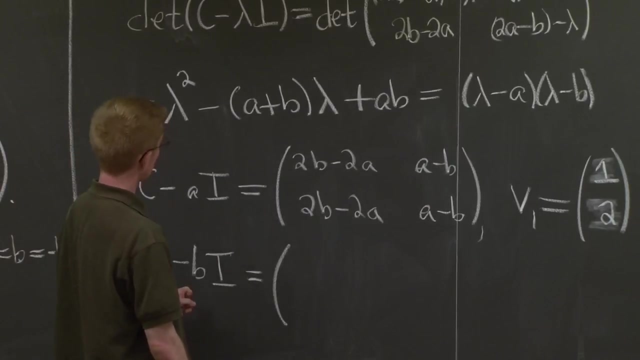 It's just 1, 2.. Good, Now, well, I guess we have space to do the second one too, Why not? So let's write out the second one also. Here we're subtracting B instead of A. We get B minus A. 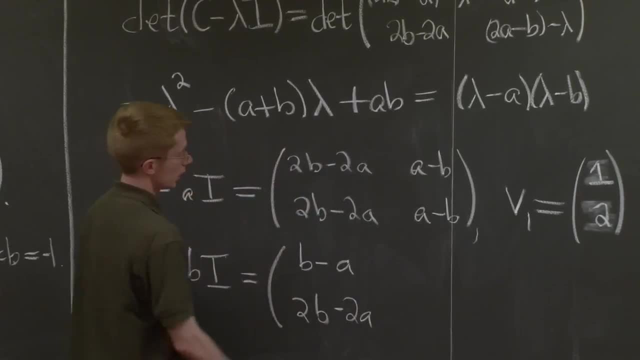 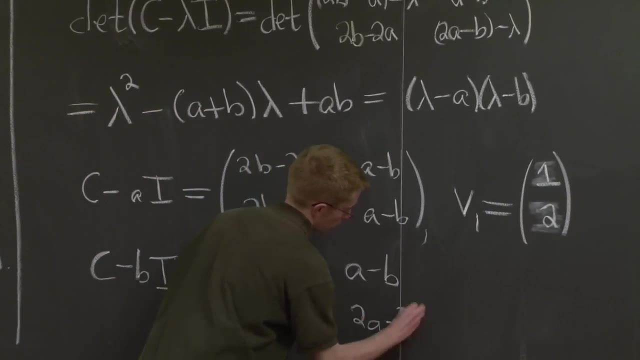 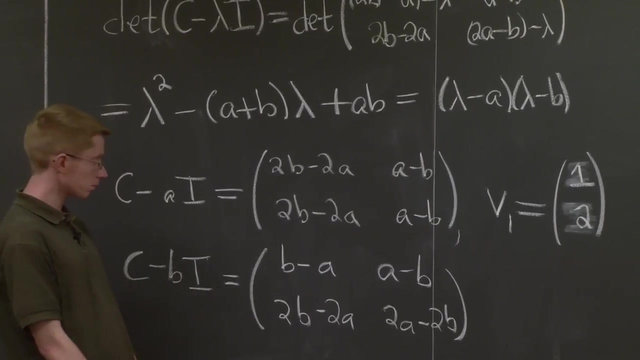 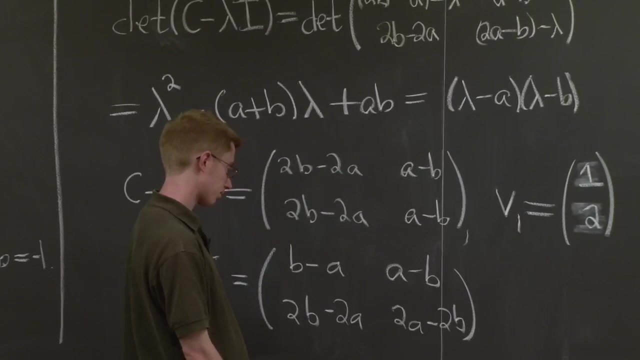 We get 2B minus 2A. We get A minus B, And what do we have here? We have 2A minus 2B. OK, So now what's in the null space of this matrix? Well, what you can see is that this column is negative 1 times. 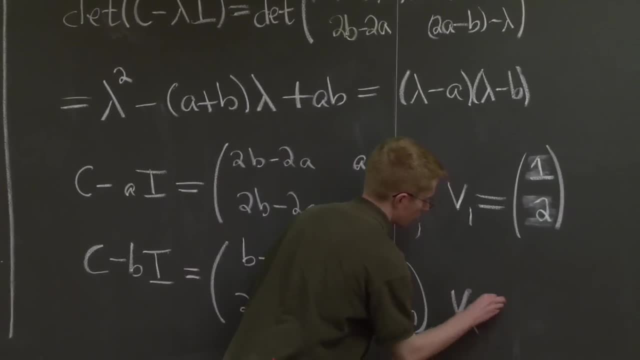 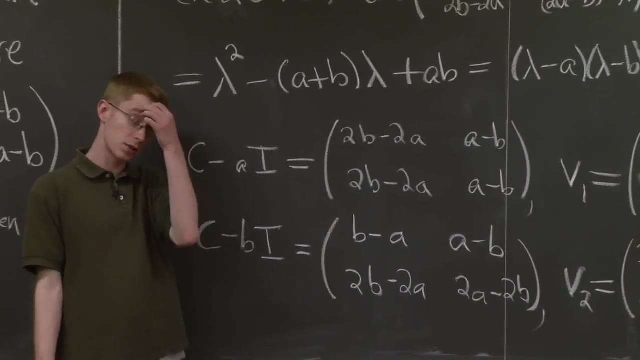 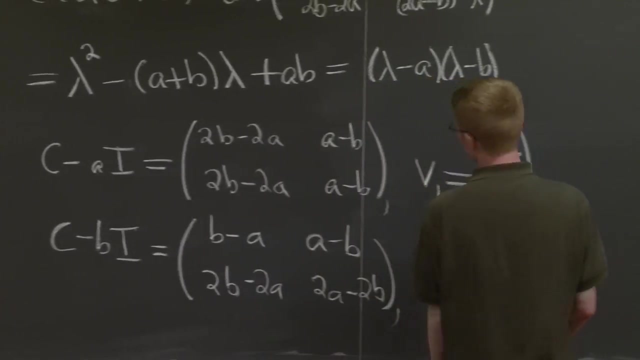 that column. So our second eigenvector is just going to be 1, 1.. And I should remind you that if you have a harder example, you can just find these null spaces by elimination, like we always do. Great, Now we have our eigenvalues and our eigenvectors. 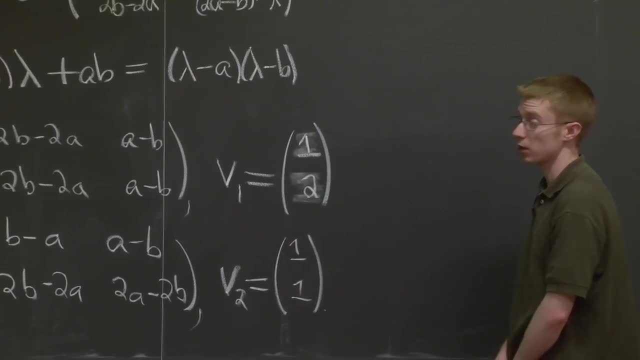 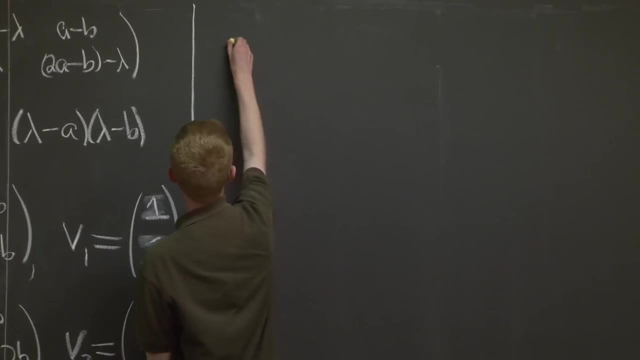 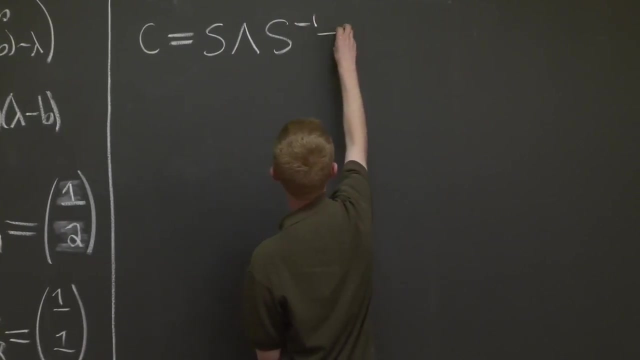 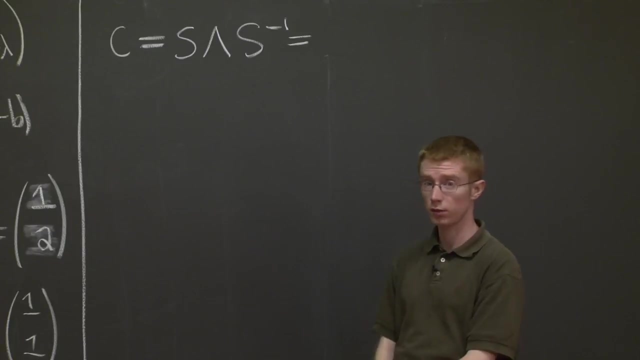 So now we can write C in a nice easy way that allows us to take powers of it. So what's that way? So that's: C equals S, lambda, S inverse. So this is just what is S. remember S's are matrix of eigenvectors. 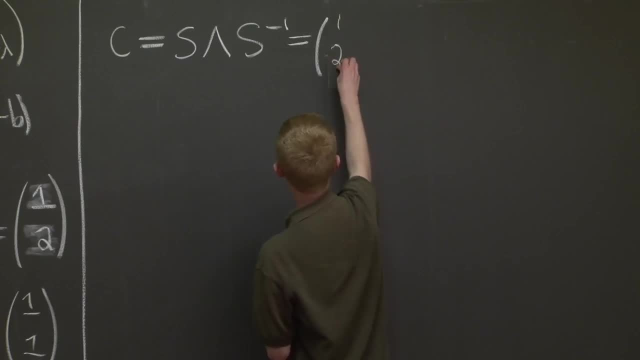 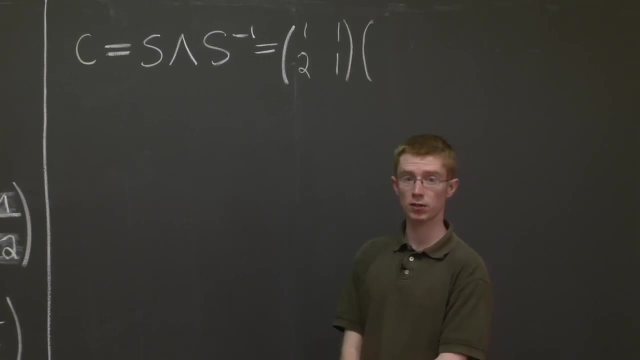 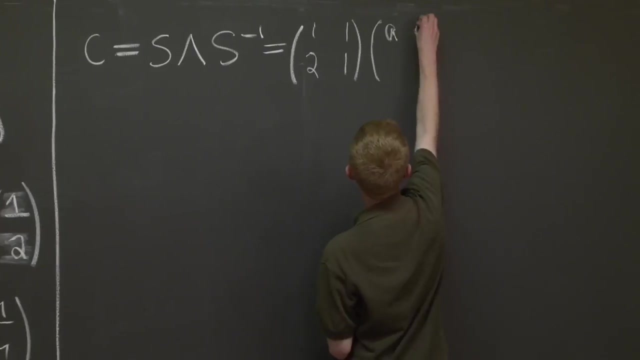 So S is the matrix 1, 2, 1, 1.. Good, Now what is lambda? Lambda is the matrix of eigenvalues, right? So it's just A and B. Those are the diagonal entries of my lambda matrix. 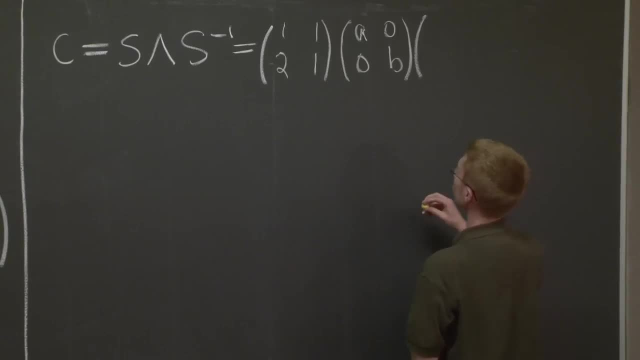 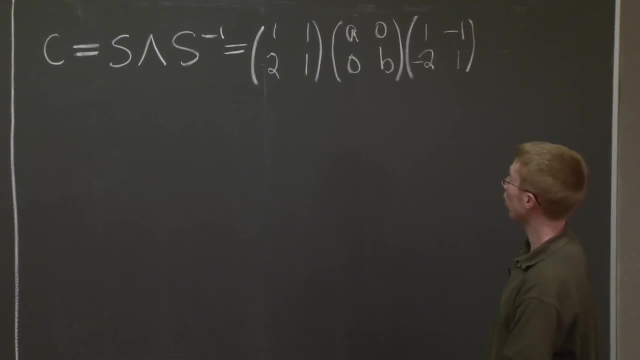 And then we just find S inverse. So we just take, We just take negative signs here And recall that we have to divide by 1 over, or we have to divide by the determinant, And the determinant of this matrix is just negative 1.. 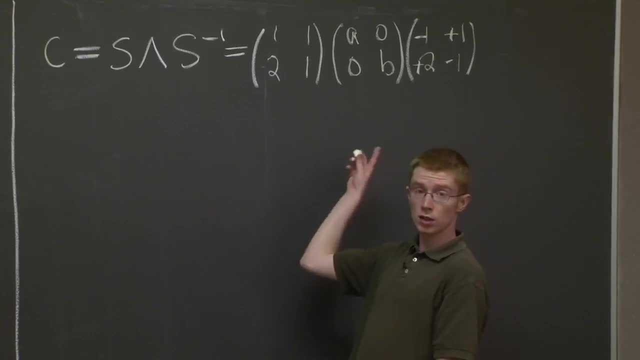 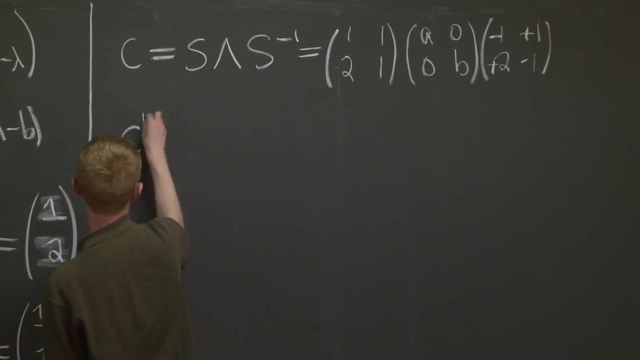 So we just change the S signs there. Good, So this is our nice decomposition of C. Now, how do we take powers of C? Well, C to the k is just S. lambda to the k. S to the k S, lambda to the k. 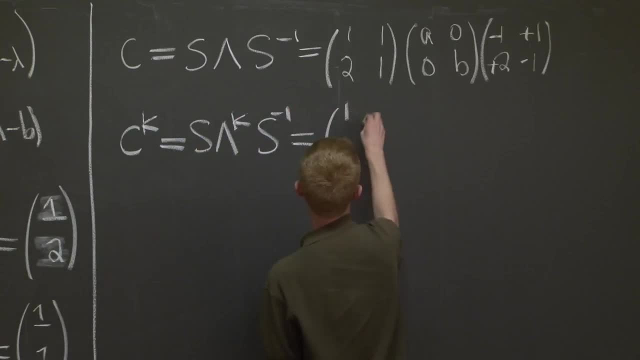 S to the k S to the k S inverse right: 1, 1, 2, 1, A to the k B to the k negative. 1, 1, 2, negative 1.. 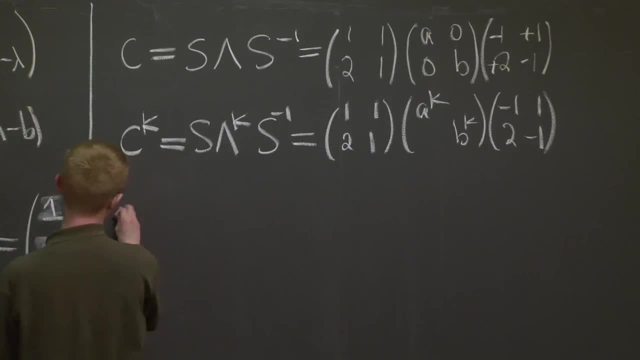 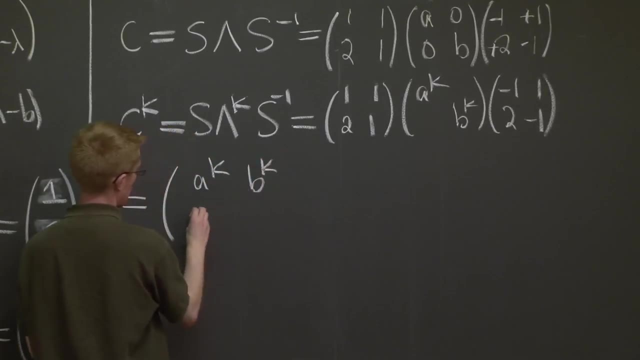 Good And multiplying these matrices together. just do a little arithmetic here- Get a bunch of powers of A and B, because we take powers of the eigenvalues. So we have here: we have 2B to the k minus A to the k. 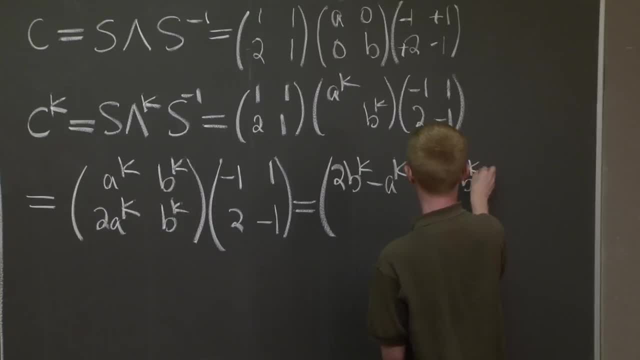 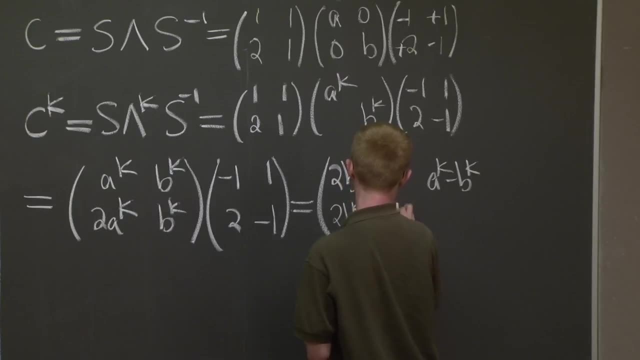 Have A to the k minus B to the k. have 2B to the k minus 2A to the k. Let's get that here. So we take the powers of the eigenvalues a to the k and finally we get 2a to the k minus b to the k. 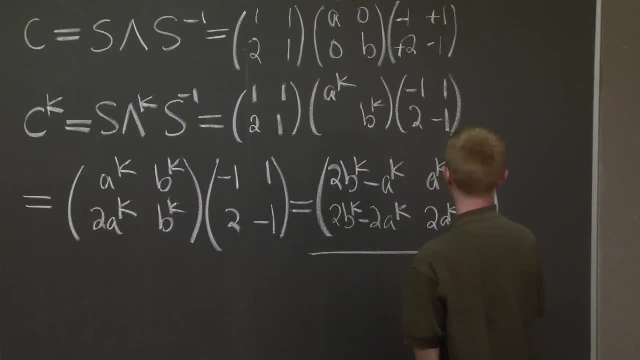 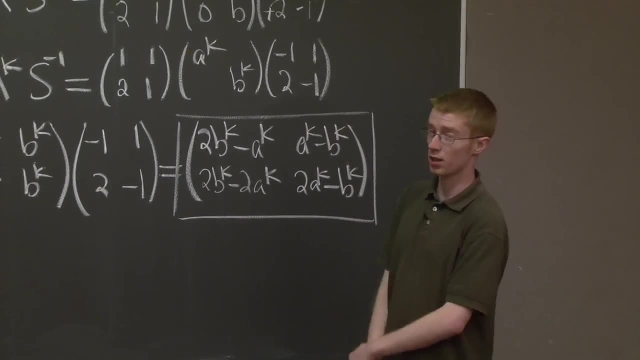 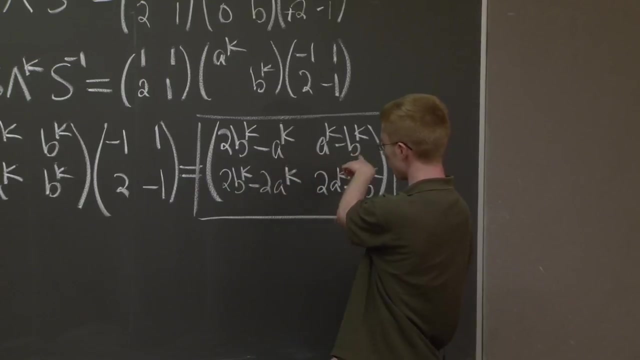 And this is our k-th power matrix. A quick check: it's always good to check your work here. Let's plug in k equals 1, and what do we get? We get 2b minus a, a minus b, 2b minus 2a and 2a minus b. 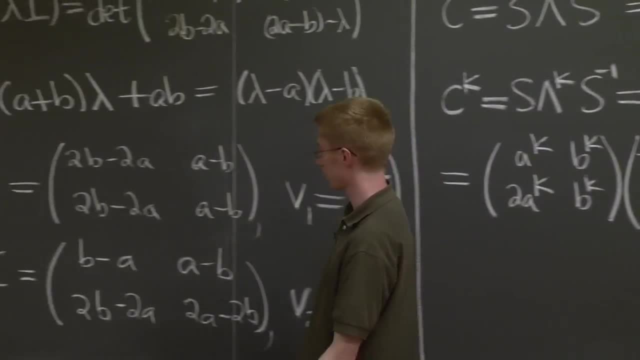 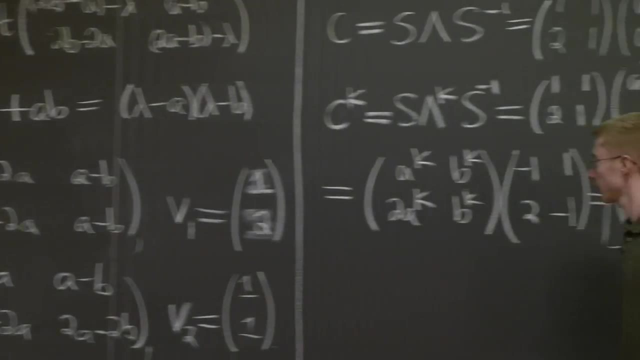 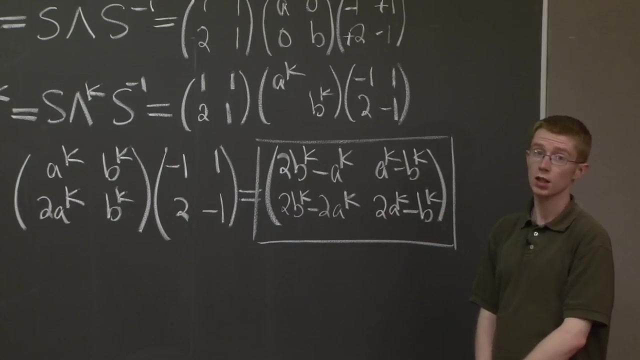 And if we can go all the way back to our matrix at the very beginning, all the way back here, that agrees perfectly with what we started with. So that's good. That means that we did this decomposition right. Good, So now we've computed the k-th power of this matrix. 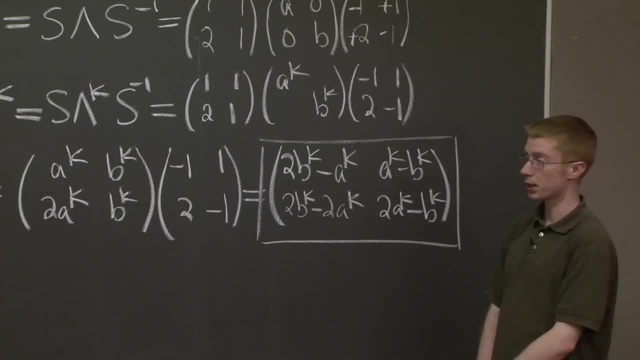 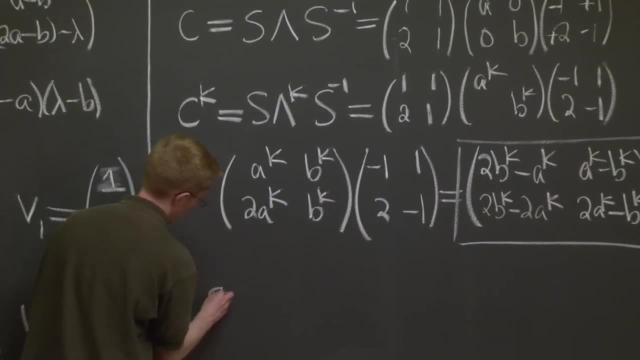 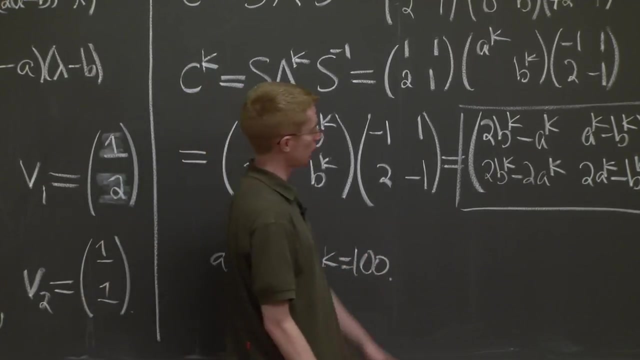 Let's do a particular example. So let's plug in: a and b are minus 1.. So a equals b equals minus 1, and k equals 100.. Then what do we get? Well, minus 1 to the 100-th is just 1.. 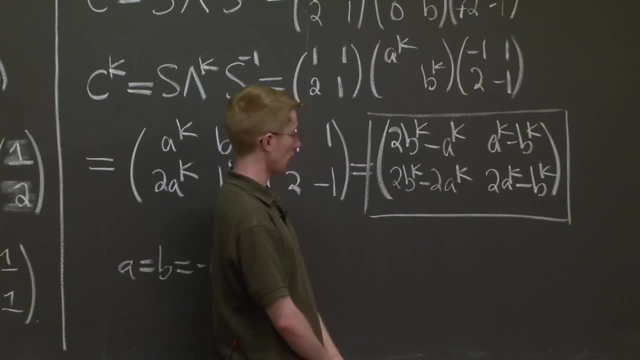 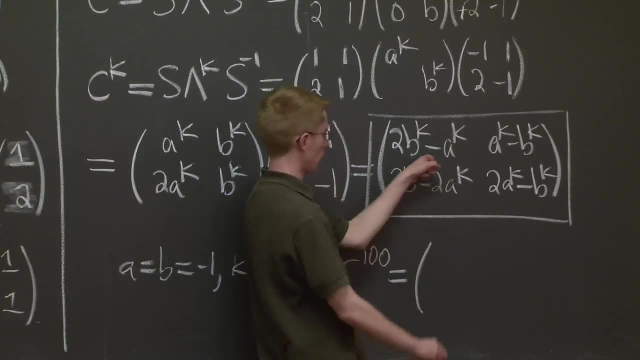 So we're just plugging in 1 for b to the k and a to the k everywhere, And we just get, in this case, c to the 100-th is just well, 1.. 0,, 0, 1..